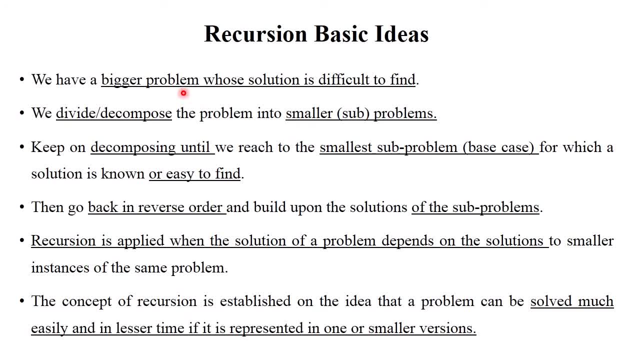 find now, at that time, what we do. we divide or decompose the problem into the smaller sub problems means main problem can be divided into the smaller sub problems and keep on decomposing until we reach the smallest sub problems. this smallest sub problems which is called as a base case, because the solution of 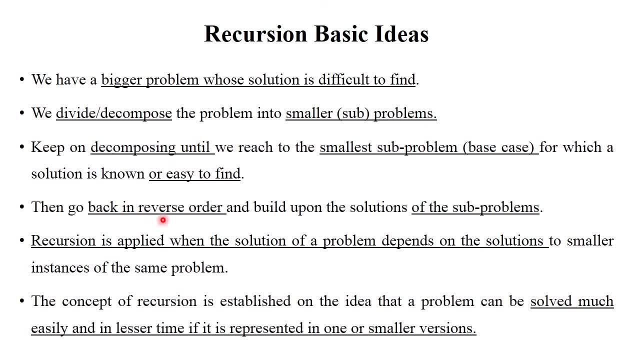 that particular problem is easy to find. then again we go back in reverse order and build upon the solution of these sub problems. clear means there is main problem is available. to find out the solution of that problem, we divide the main problem into the smaller sub problems and after that we solve each and. 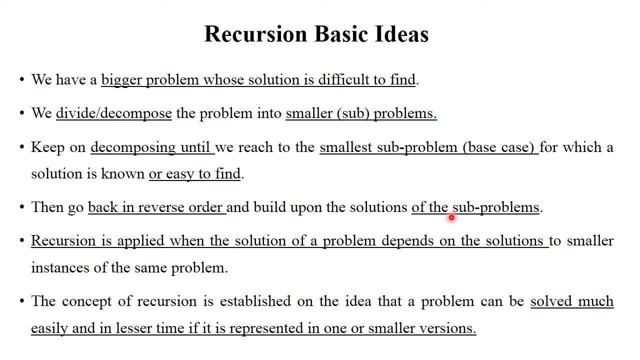 every smaller sub problems and go into reverse back. means smaller subproblem is again integrated to solve the main problem. clear, this is the concept of recursion. recursion is applied when the solution of problem depends on the solution to smaller instance of this same problem. the concept of recursion is established. 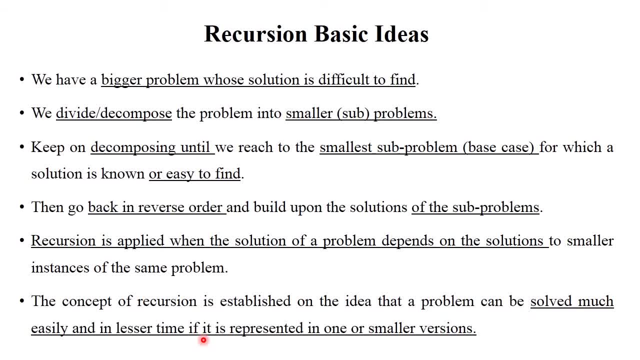 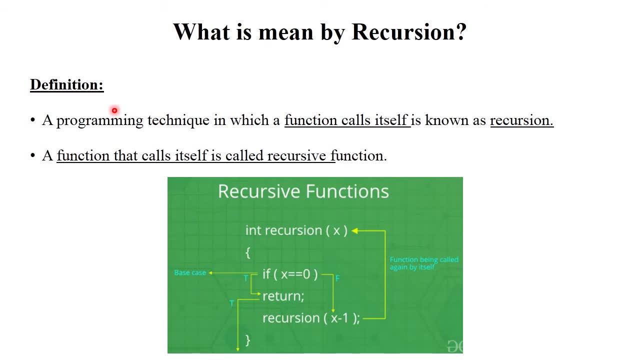 on the idea that problem can be solved much easily: laser time and, if it is represented in one or smaller versions, clear. so this is the idea or concept behind the recursion. so let's see what is meant by recursion. so here, definition of recursion. recursion is a programming technique. 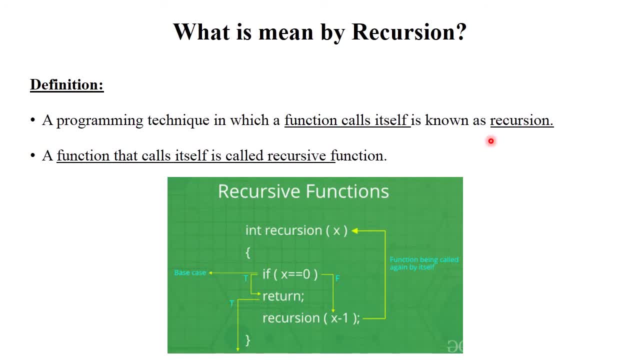 in which function call itself is known as recursion. you must remember: function call itself a function that call itself is called as recursive function. now see here: this is the structure of recursion or recursive function where function is recursion integer. recursion integer is data type, recursion is the function and we pass the parameter x clear in that function. 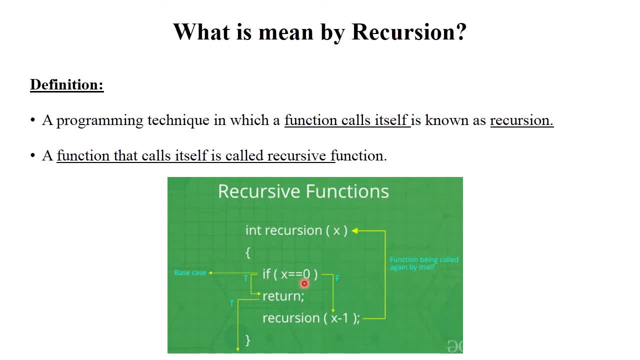 there is. if condition is used: if x exactly equal to 0, then return. but if this condition is false, then go to the next step. that is recursion. x minus 1. see here in recursion function. we call again recursion function means this: x minus 1 goes to here again we call recursion function again we. 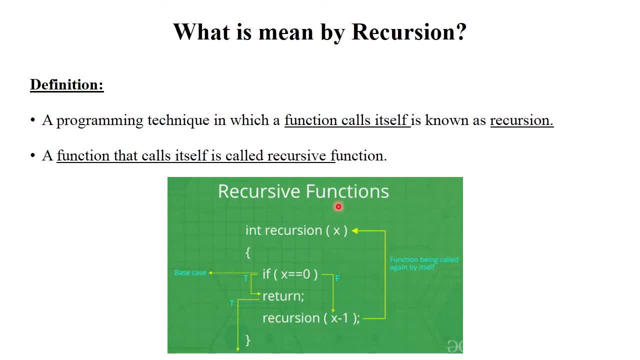 goes to here: again we call recursion function and again we goes to here: clear it means that function call itself, this recursion function call itself again. so this is called function, being called again itself. this is the concept of recursive function, understood, okay. next see here i will take one example of recursive function. 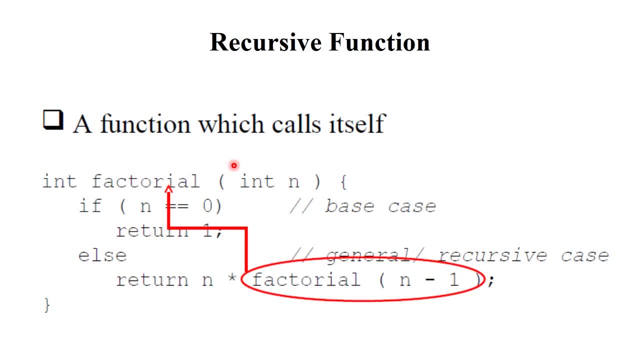 the main or main function or main example of recursion is factorial. we know that concept of factorial right, so see here: this is the logic behind the calculation of factorial. so recursive function means function calling itself. see here: integer, factorial. integer n, it's the data type, factorial is a function name. in this function name we can pass the one parameter. 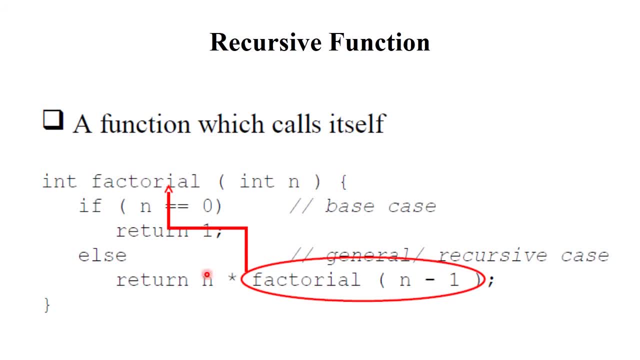 that is integer n. in fact, ins переж asalis n. it is go to here now, in this factorial function, if else condition is used, if an exactly equal to zero, then it's return one, okay. but if this condition is false then it moves to else part and what else in else path- Britain- and into factorial and minus 1 now. 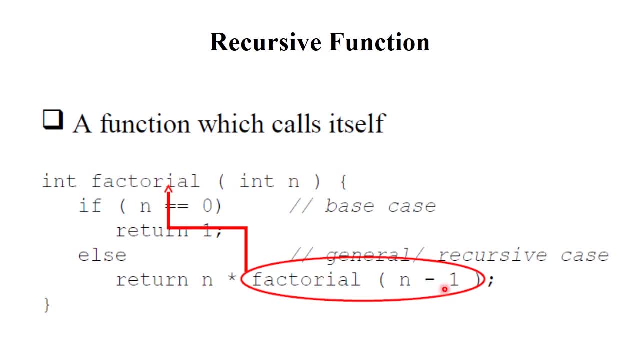 see here factorial function again call factorial function means function, call itself clear and at this value stored into this n again goes to else loop, again this value is calculated, again stored into this n means this is called recursive function, clear. so let's take one example with programming of recursive function now 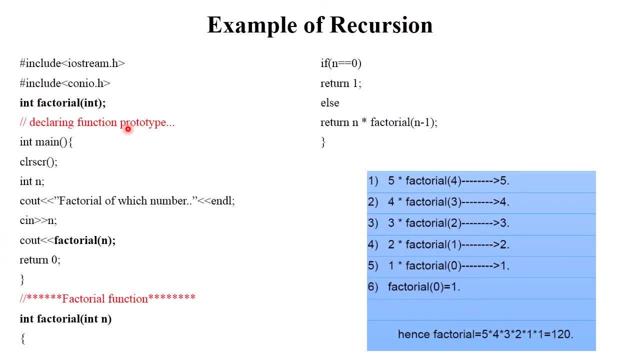 see here. this is just general or basic program of factorial. okay, the program is all already in C++. now see here: program always start with header files. hash include iostreamh, hash include conioh, the, all the data types like cout. cout is used for printing purpose, cin is used for read purpose, so 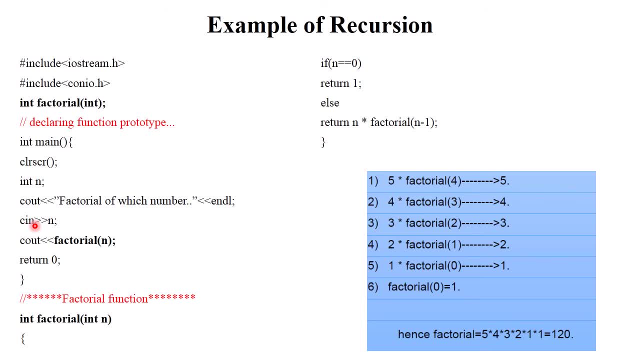 these all are built-in keywords and this built-in keywords are stored into this header. files like iostreamh, conioh, etc. clear. after that program always start with main function: okay and the function name is factorial- integer, factorial. okay and the function name is factorial- integer, factorial. 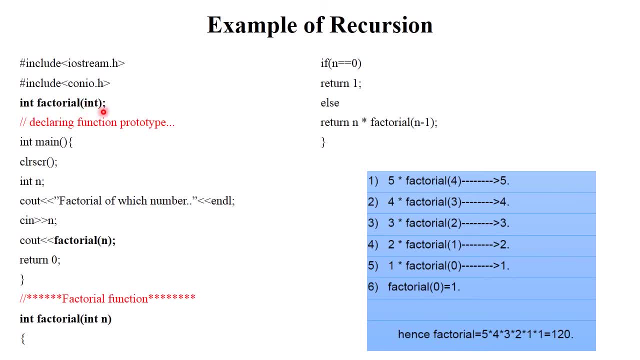 integer factorial and we pass the element always in integer type. so this is the declaring function prototype. now see here when we implement a program or execute the program. so first line is factorial of which number? before start the programming I will tell you factorial means. if we calculate the factorial of 5, then 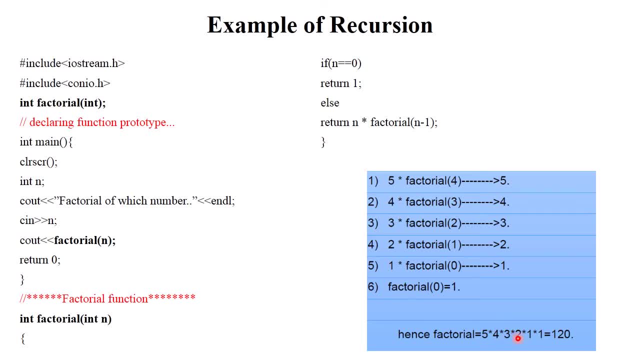 factorial of 5 is 5 into 4, 4 into 3, 3 into 2, 2 into 1, equal to 120. factorial of 4 is means behind numbers like 4 into 3, 3 into 2, 2 into 1. factorial of 2 is 2 into 1. means 2 clear. 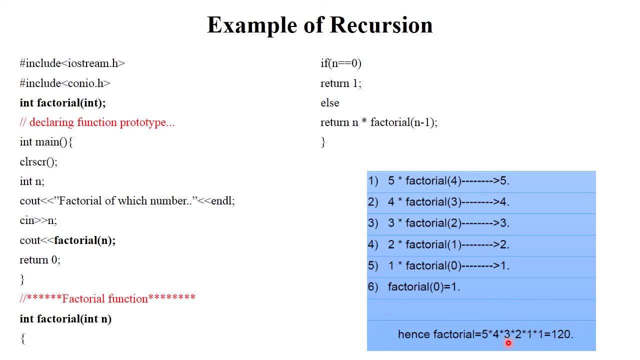 this is the concept of factorial means: recursively call each other. okay. now see here when we, when you execute the program, the first line is: see out factorial of which number. if you need to calculate factorial of 5, okay, so you enter 5, so the command line or for reading purpose, we use C in keywords, so n equal to 0. 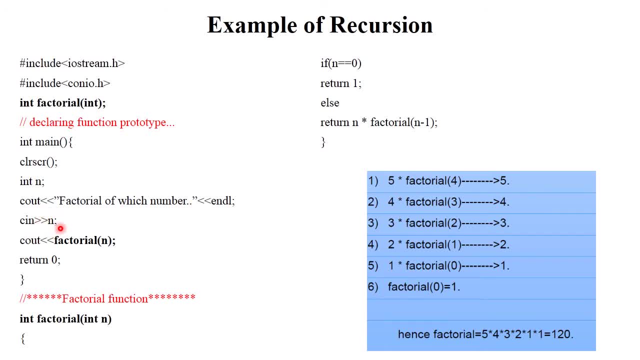 equal to 5 means you need to calculate factorial of 5. now see out factorial of 5 and equal to 5. then this called to this function. okay, function all always define in after the main function. clear now. in this factorial function we implement the logic of factorial, see here: 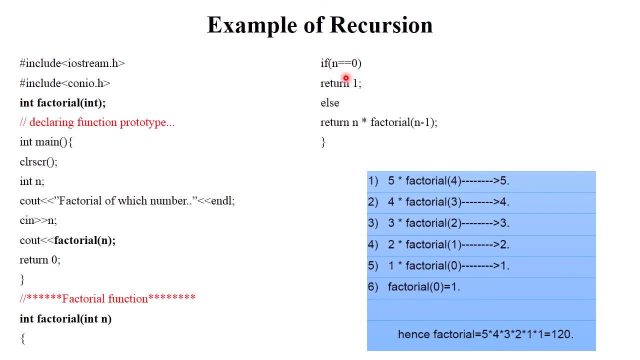 if n equal to 0, our value is n equal to 5. so if n exactly equal to 0, no condition is false, so it moves to else part. if condition is true, then the return one. if condition is false, then it move to this else part. so this is just simple logic of factorial. 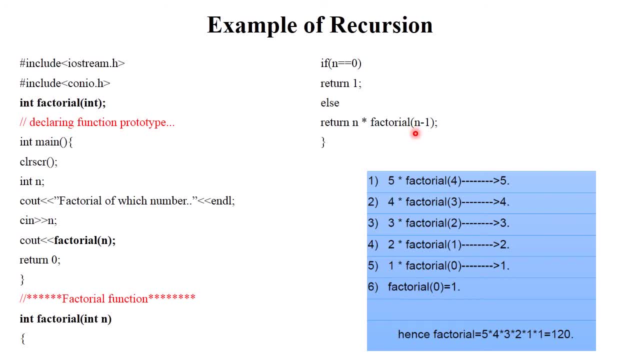 see now: n value is 5, so n equal to 5, 5 into 4, n minus 1, 4. now 5 into 4 and this value goes to here again. this function is executed at that time. 5 into 4. this value is stored here. and 4 minus 1: 3 then. 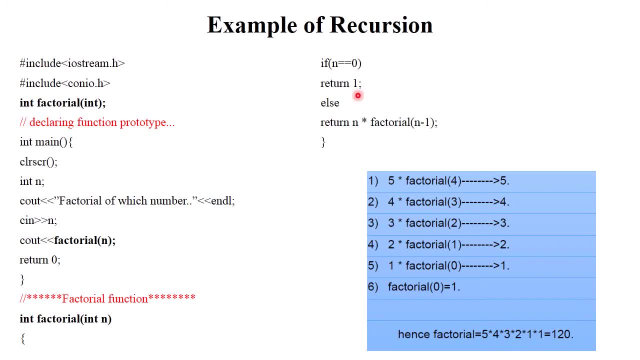 again. this function is executed in this way recursively: 5 into 4, then 4 minus 1, 3, then 3 minus 1, 2, 2 minus 1, 1. in this way it completely executed clear. in practical session we will implement this program in more detail way. okay, at that time you need to understand just.